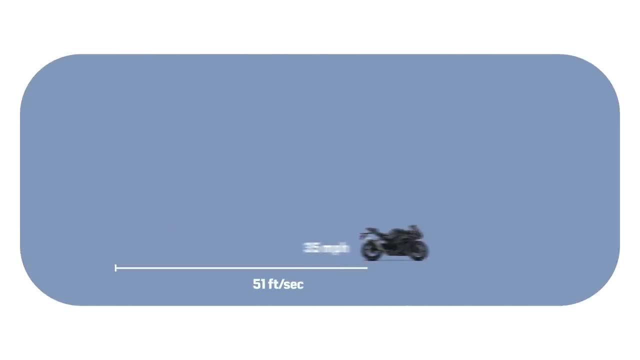 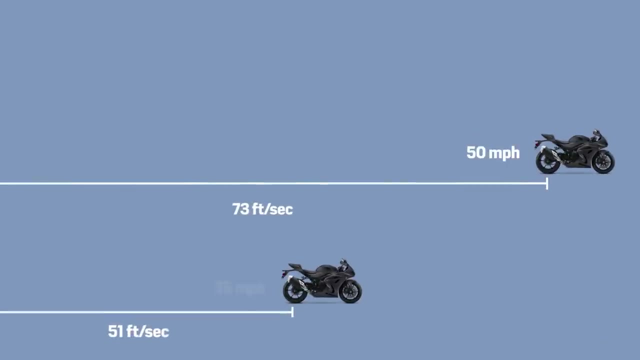 consequences: 35 miles per hour equals 51 feet per second, And 50 miles per hour equals 73 feet per second. So when you go 50, and a 35,, you have 22 fewer feet to stop per second, Meaning far less time to react if and when something goes wrong. That's a big deal because when motorcycle fatalities involve another vehicle, 43% of the time it has a car turning left into the path. Less speed, more intuitive anticipation and faster reflexes on the brakes would help improve the odds of survival for the motorcyclist. 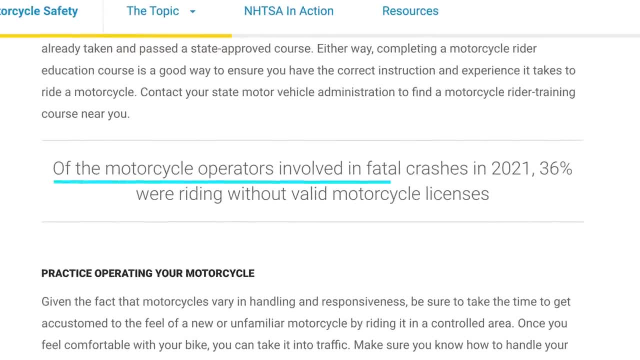 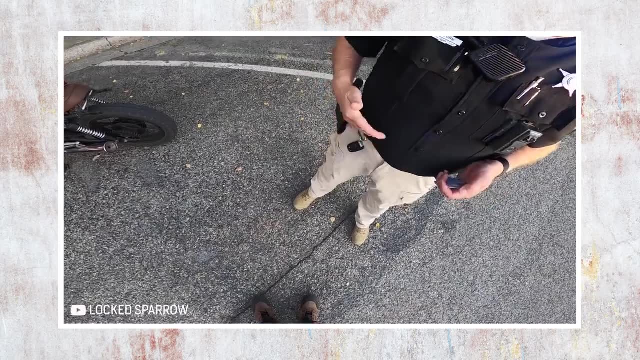 Speaking of rider skill, records show that 36% of all motorcycle fatalities involve a rider who has no motorcycle license. According to the computer, you don't have a motorcycle license. Because you don't have a license, I can't let you go. 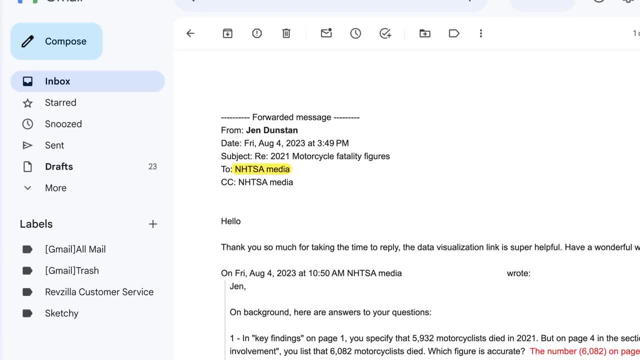 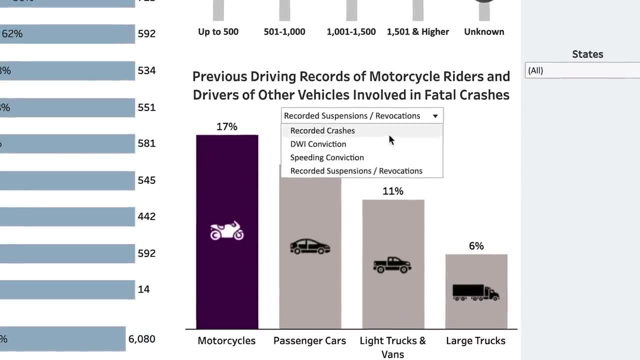 Now, to be fair, this data is somewhat incomplete. NHTSA does not report how many of these riders had a learner's permit or not, or how much riding experience they had, regardless of license status. For all we know, many of these riders may have years of seat time, but never. 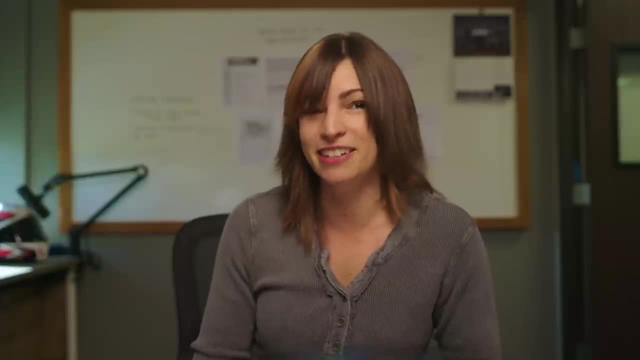 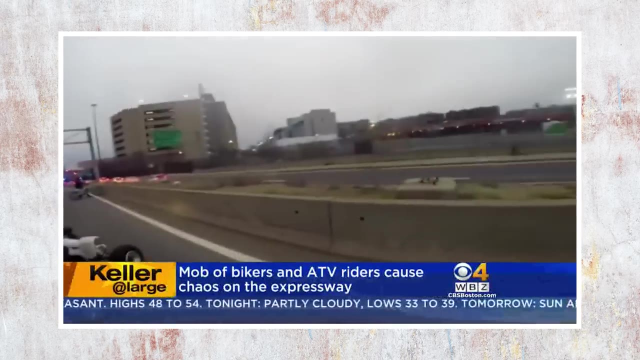 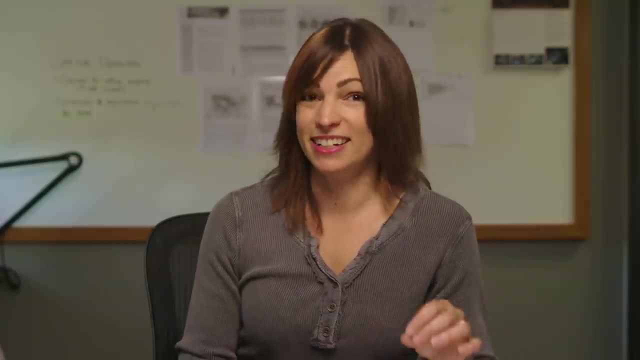 bothered to get a license or had their license suspended. So it's possible and even likely that poor decision makers, rather than exclusively new riders, are responsible for this high rate of unlicensed fatalities. And that begs the question: what other data points in these statistics aren't telling? 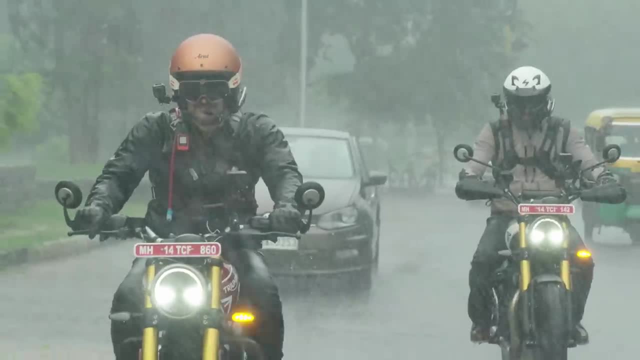 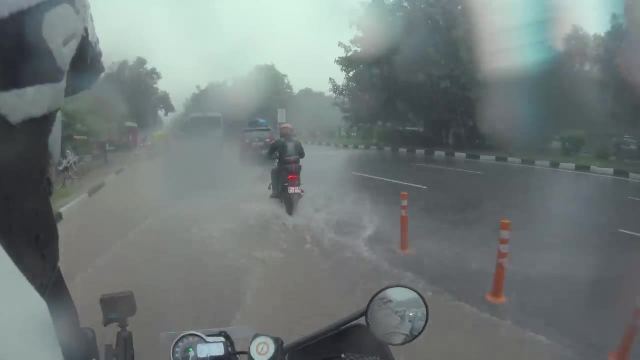 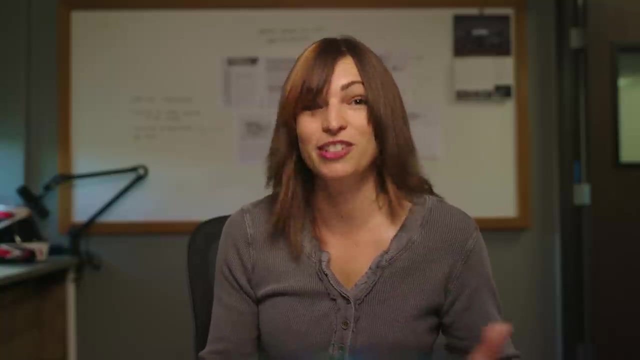 us the whole story. For example, did you know that only 2% of all motorcycle fatalities happen in the rain? Is this because wet conditions aren't dangerous? Or is it because the vast majority of riders choose not to ride in the rain? 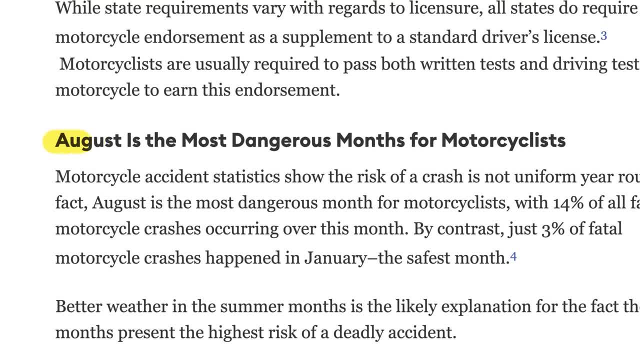 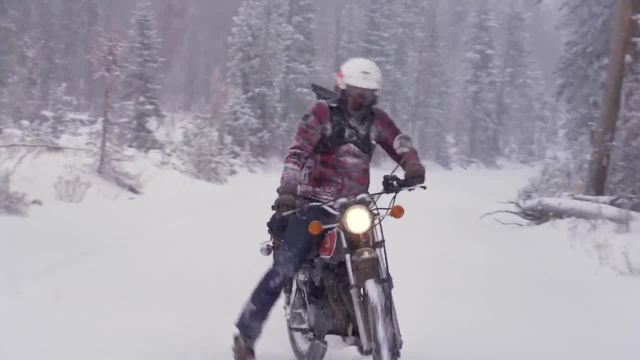 And were you aware that, statistically, the most fatal month of the year for motorcyclists is August, while the least fatal is January? But again, riders avoid bad weather, so it makes sense that there are fewer riders on the road in winter than there are on the road. 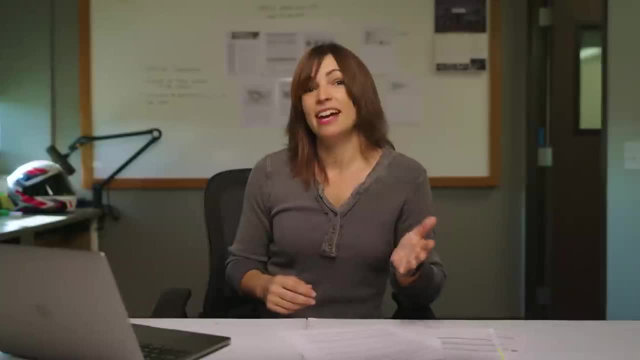 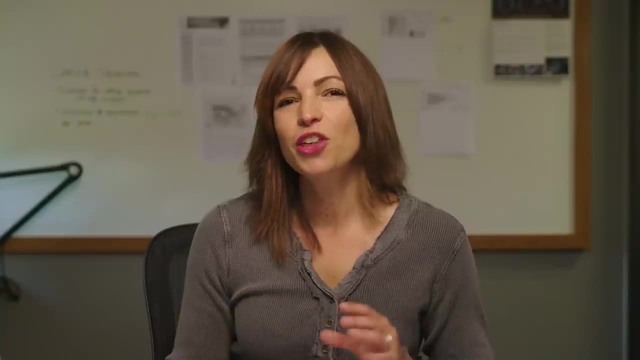 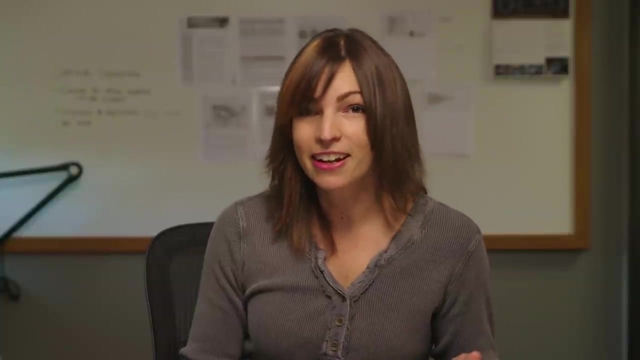 What this all means is that context is important when we look at the data. We have to be picky with which statistics are going to inform rider habits. The good news is, if we can better understand where and how these accidents are occurring and identify the common trends, then we have a chance. 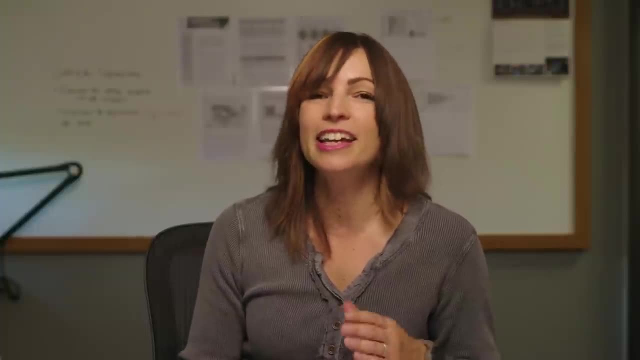 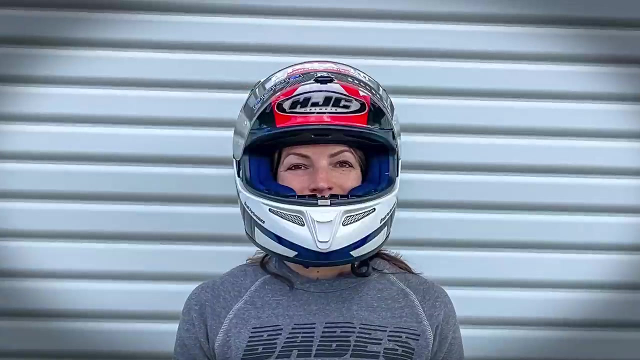 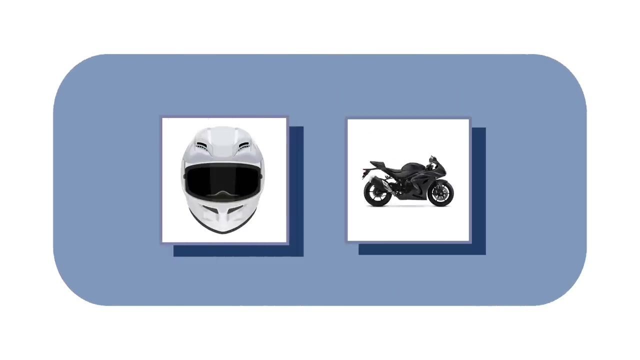 A chance to change habits, be more aware and keep more riders safe out on the road. So, first and foremost, protect your head. By just putting a helmet on, you improve your odds of avoiding a fatal crash by 61%. Second, don't drink and ride.